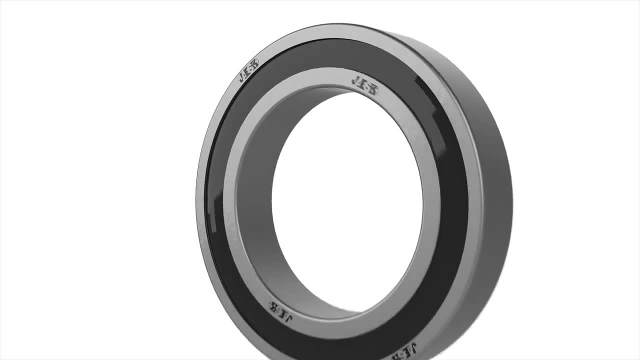 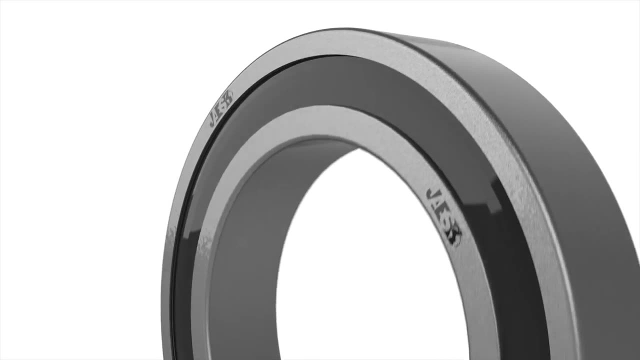 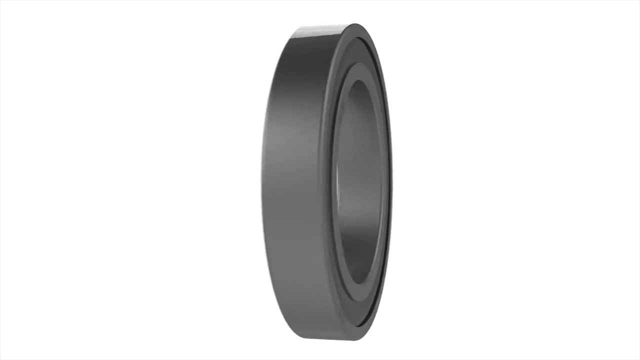 be made of plastic preventing liquid infiltrations. They are placed in specific locations between the two rings so that they can protect the balls and the cage from external agents. At the same time, they can retain oil or grease inside the bearing, keeping it lubricated for its entire life cycle. 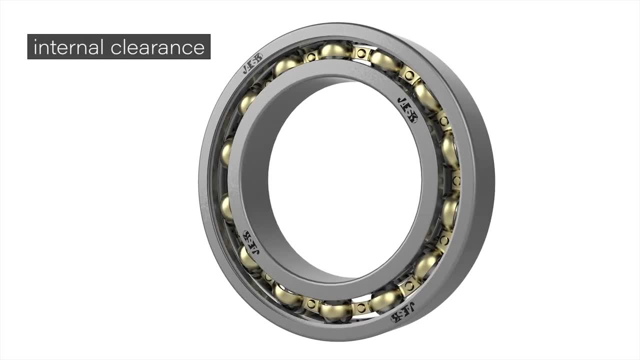 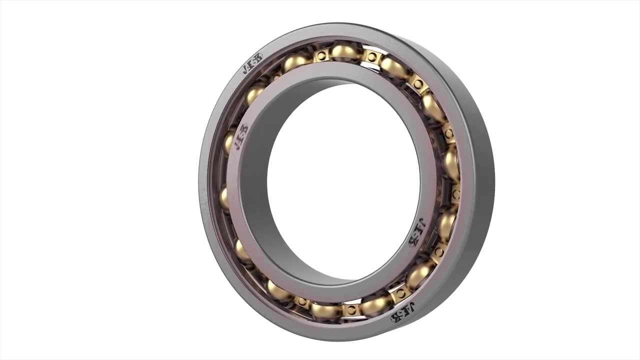 In order to work correctly, bearings need a certain radial and axial clearance so that, when they reach the working temperature, their thermal expansion won't lead to over-tightening, which would cause the bearings to wear or, in worst case, even a seizure. 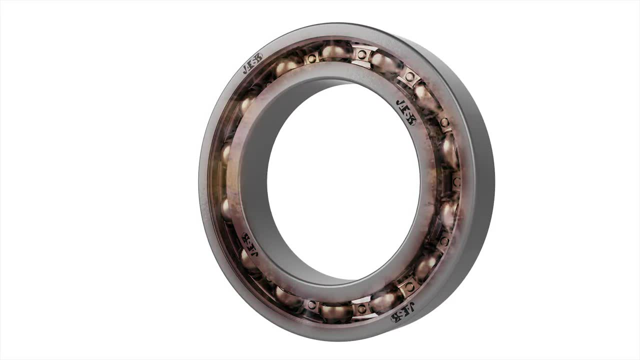 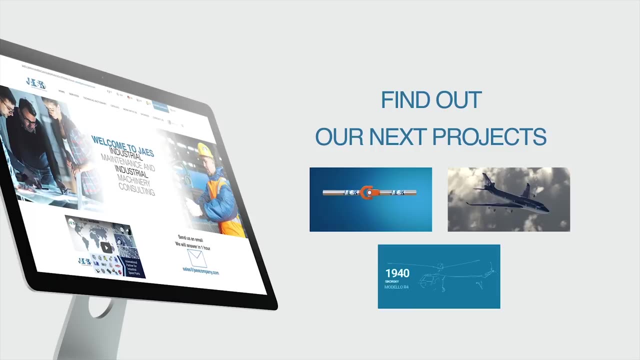 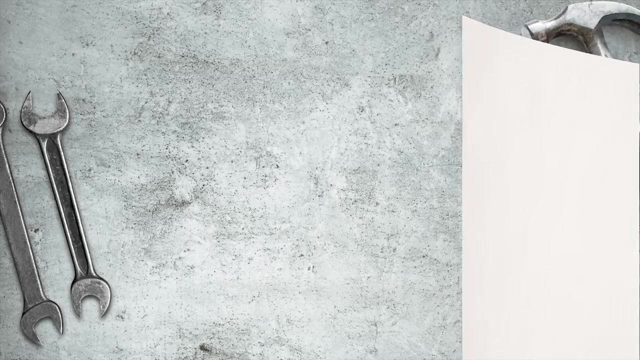 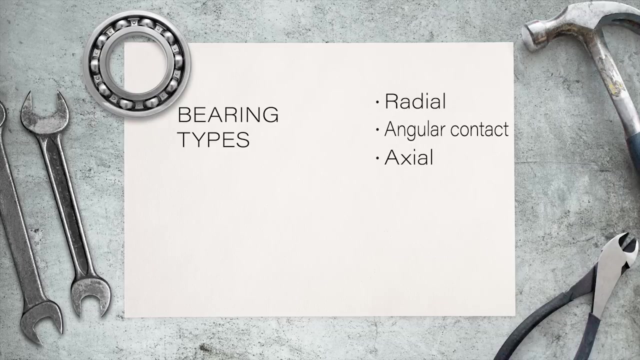 There are many different types of bearings, but the three main categories are radial bearings, angular contact bearings and axial bearings. At the same time, rotary bearings can be divided into ball bearings, radial bearings and axial bearings. The three main categories just mentioned differ according to load direction. 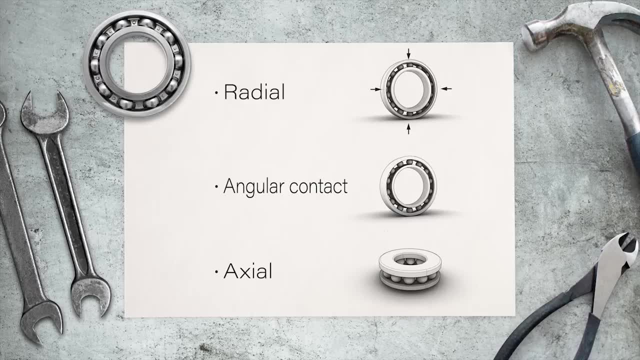 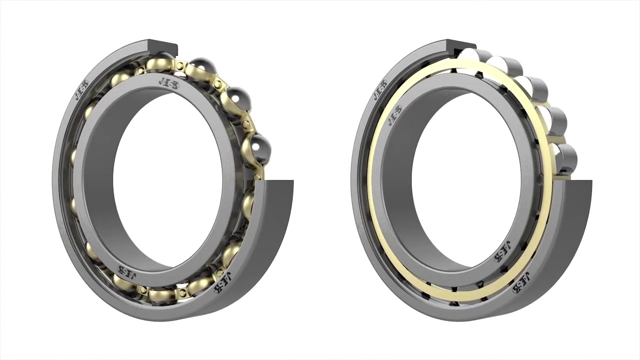 So radial bearings are used to withstand forces which are perpendicular to the axis. Angular contact bearings are used to withstand both perpendicular and axial loads, And axial bearings are used to withstand axial forces. The rotary components of the rolling element bearings make the movement easier. They are balls, as shown before, but also rollers placed between. 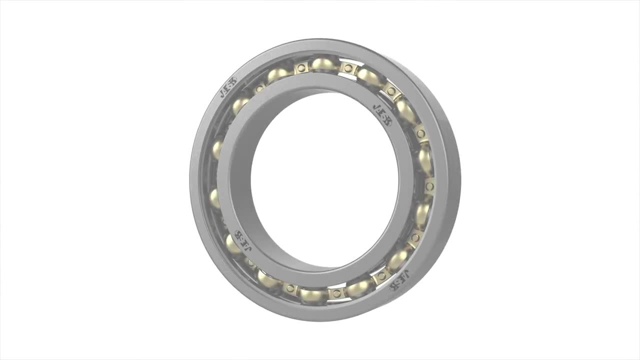 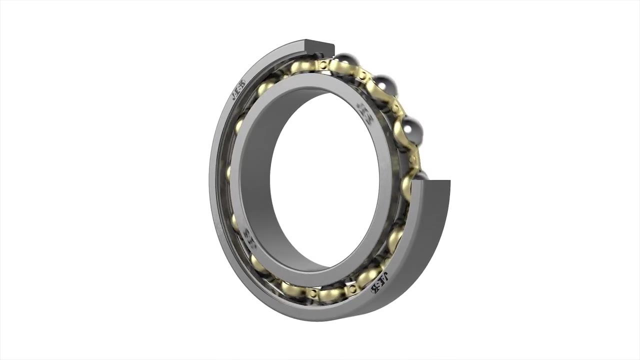 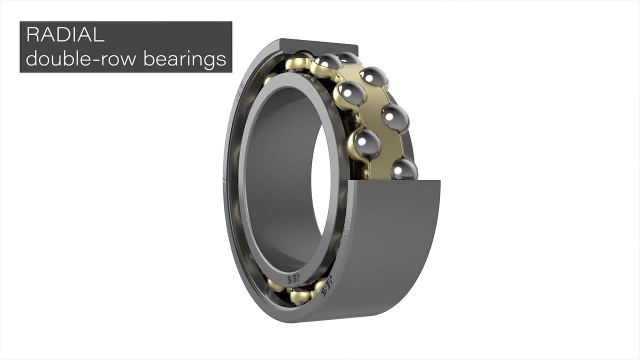 the fixed part and the moving part. Ball bearings are among the most used bearings. The radial ones can be classified as single-roll bearings- the most common type- or double-roll bearings, which can withstand high radial loads. Among the radial ball bearings, we also find the self-aligning bearings. 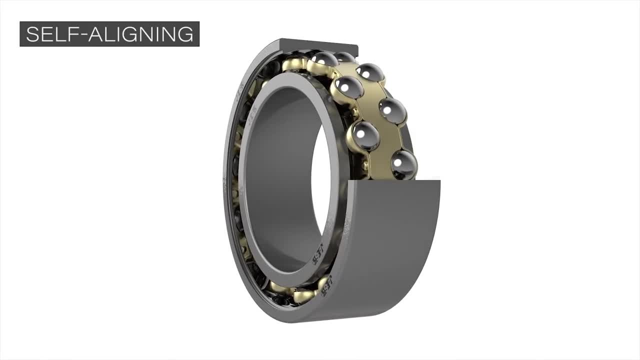 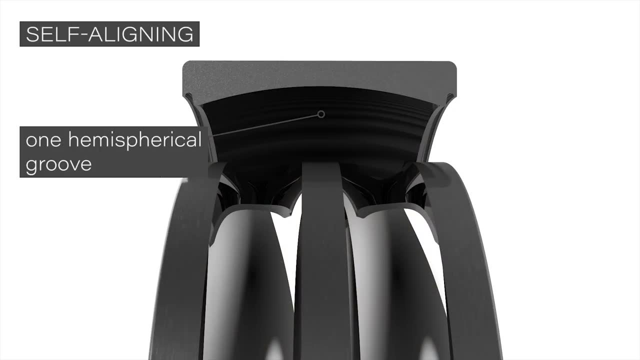 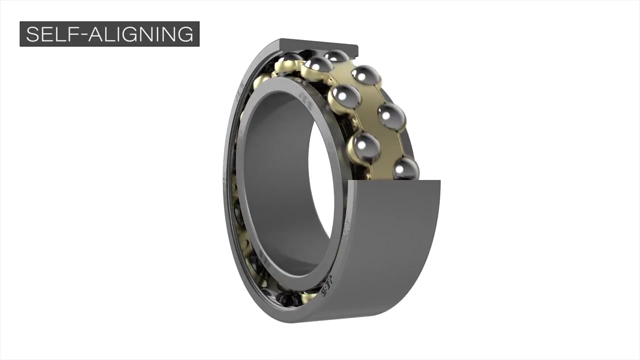 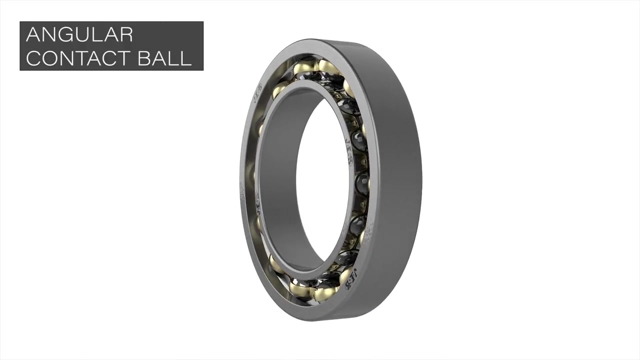 that have two rings of ball bearings. This type has an inner ring with two grooves placed side-by-side, while the outer ring has only one hemispherical groove. This system allows the inclination of the two rings' axis during the functioning. There are also angular contact ball bearings that have either one or two rings of spheres. They 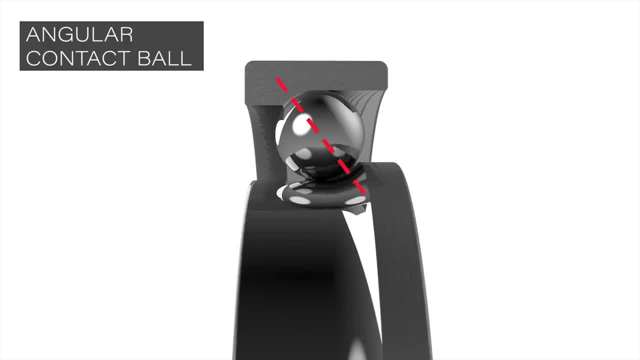 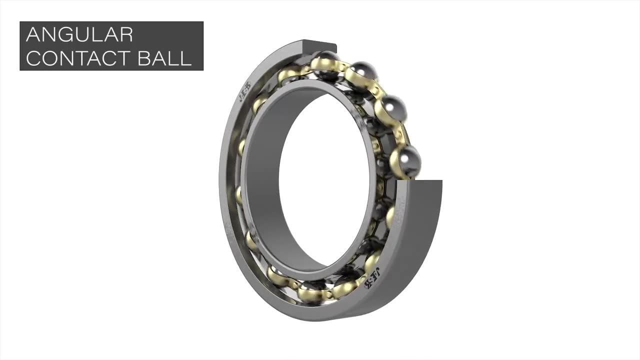 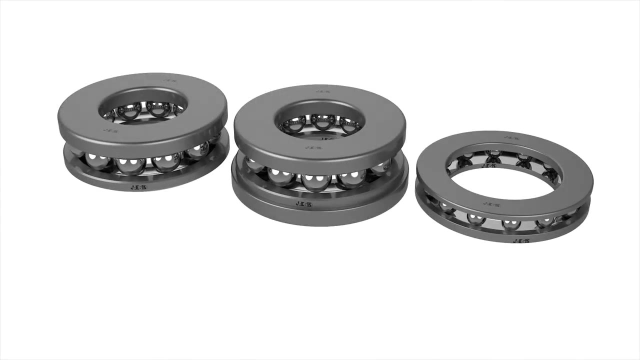 typically have an oblique position respective to the axis of rotation of the load line passing through the contact points between the balls and the rings. They can withstand higher radial loads and axial forces. Finally, it could be noted that all these varieties have an axial configuration. 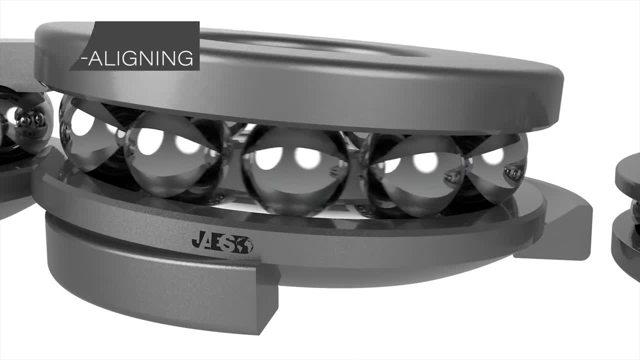 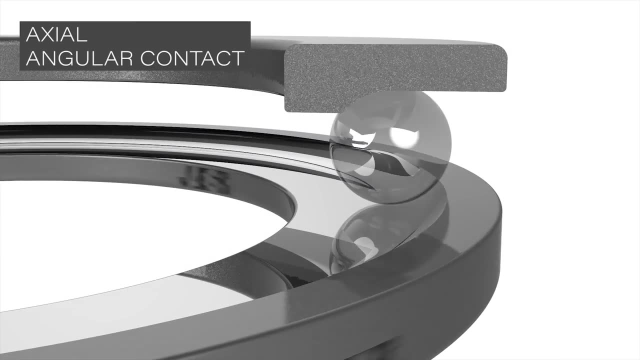 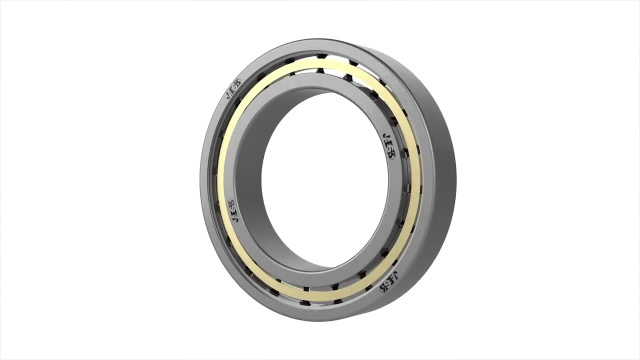 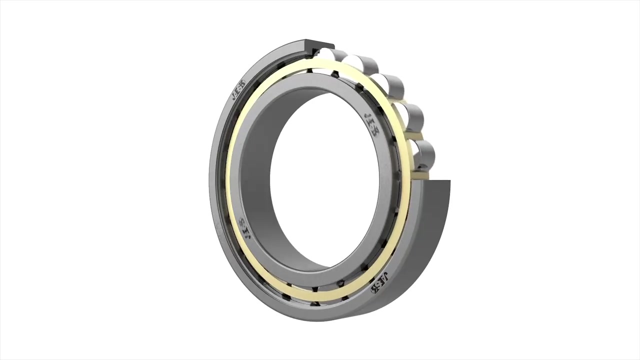 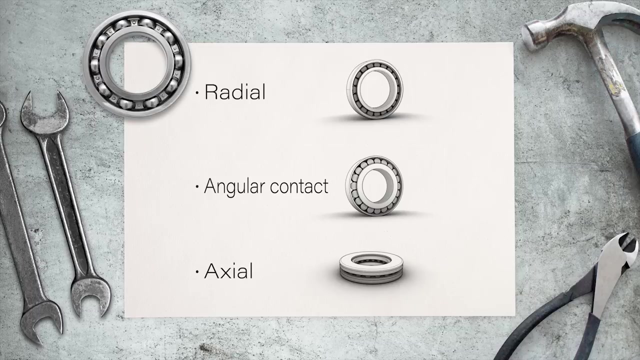 in order to withstand a mostly axial load. They are also called thrust bearings. Another major type of rotary bearings are the so-called roller bearings, used when very high accuracy is required. They have the same categories: radial, angular contact and axle bearings. 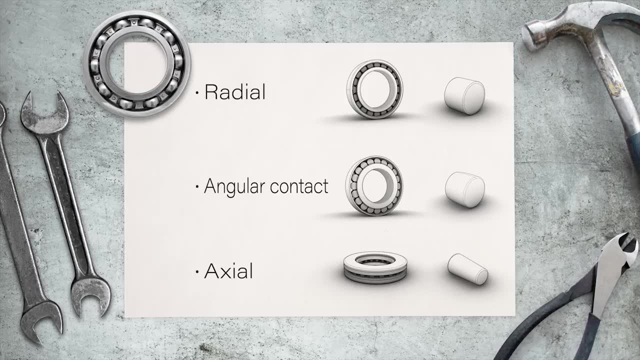 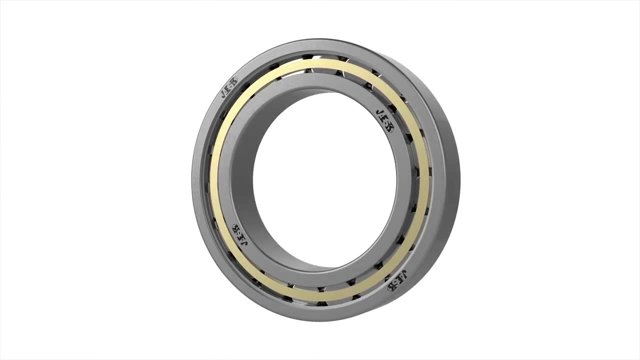 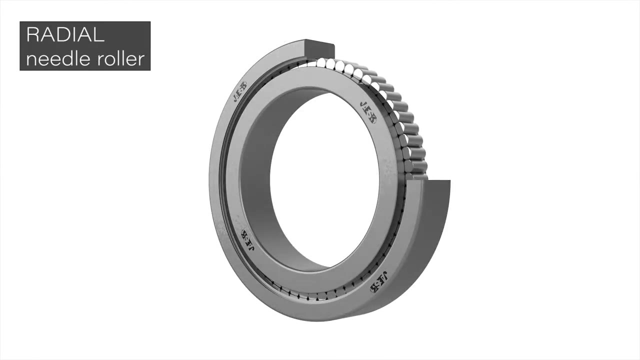 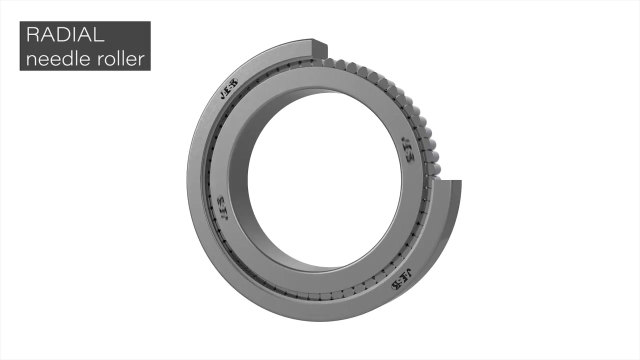 But roller bearings have different shapes depending on the type. This is another difference between these and ball bearings. Radial bearings with cylindrical rollers are the most common type. If they have small rollers, they are called needle roller bearings and thanks to their compactness, they are used when space is limited. 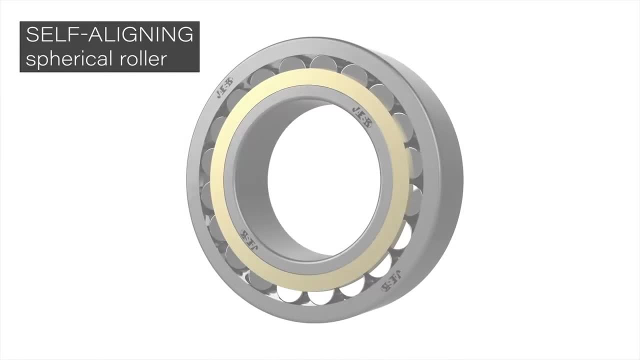 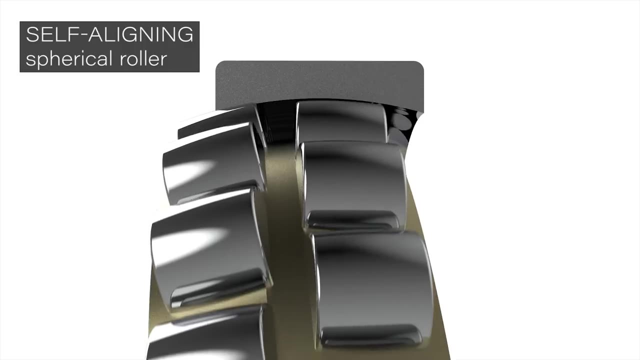 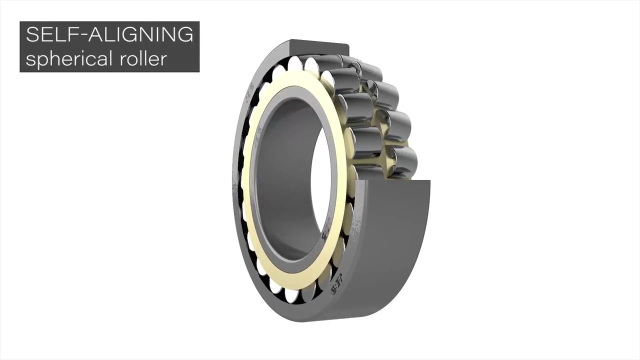 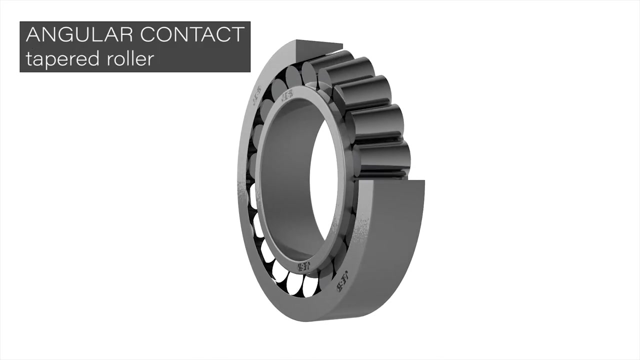 They can only withstand radial loads. There is another variety, spherical roller bearings, which have cask-shaped rollers in order to allow inclining the rotation axis of the two rings. Tapering roller bearings are an oblique version and are used in case of combined load. 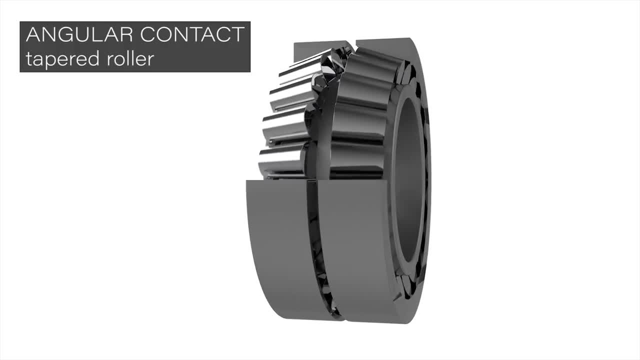 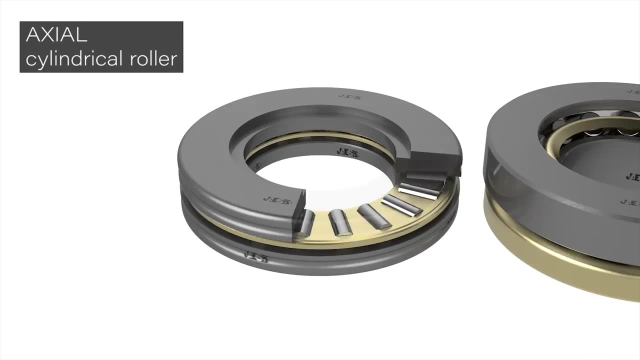 This type of bearings are generally used in pairs and they usually have inverse taper. Inverse taper bearings are usually used in pairs. Inverse taper bearings are used in pairs, and they are usually used in pairs. All of these varieties can also have axial configuration. 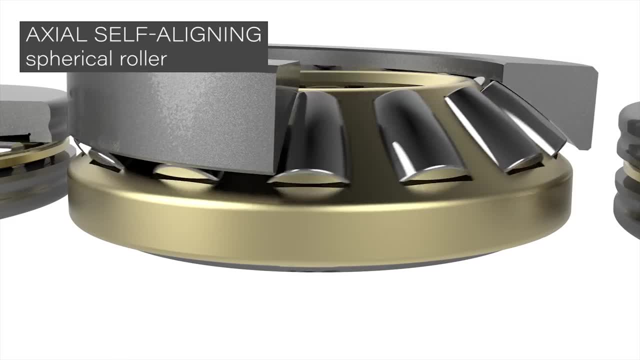 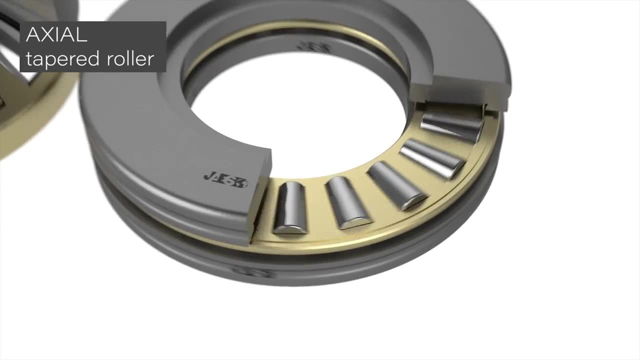 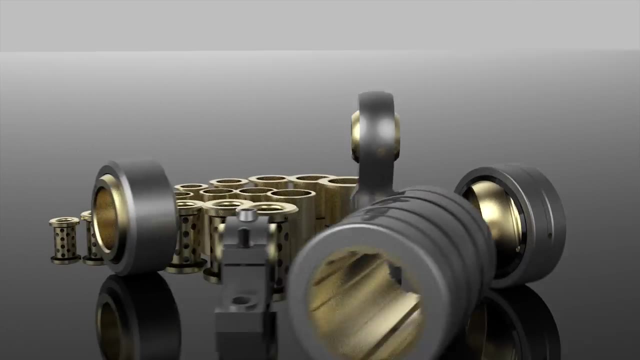 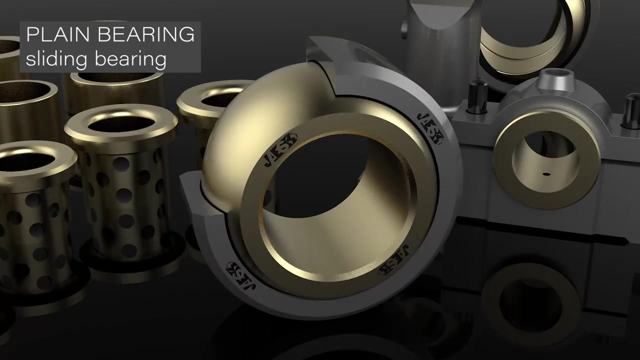 in order to mainly withstand an axial load. They are also called thrust bearings. There are many types of bearings. The most common ones are plane bearings, also called sliding bearings or slide bearings are made of two different parts. They don't have rotary elements. 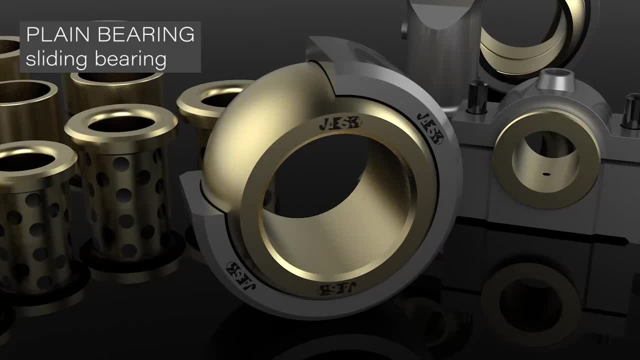 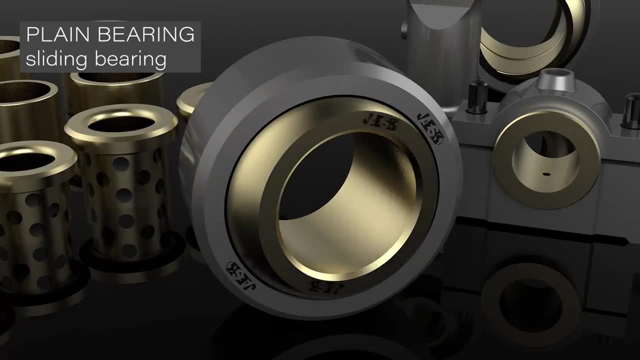 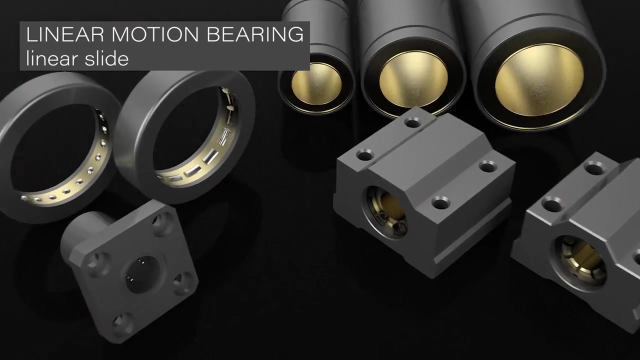 In fact, they work thanks to a thin, porous bronze foil which is covered by a layer of Teflon. The foil is placed between two elements of the bearing. These bearings are built to withstand high loads and they can also bear misalignment. Linear motion bearings are designed to provide 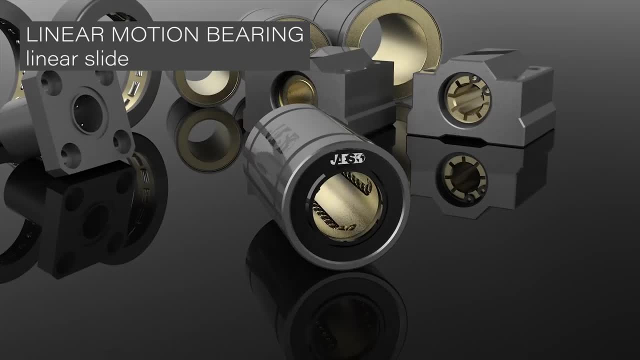 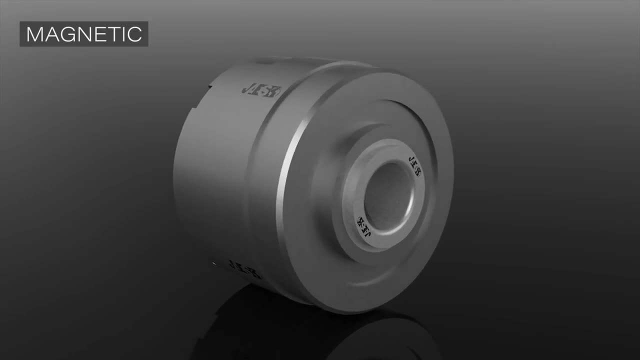 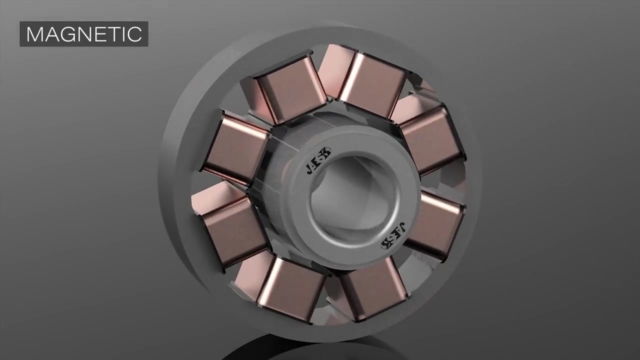 movement in one direction. They are usually called slides, And there are both linear ball bearings and linear roller bearings types: Magnetic bearings substitute rotary elements thanks to a magnetic induction, which allows them to be frictionless and avoid lubrication. As a result, they are very efficient in every condition. 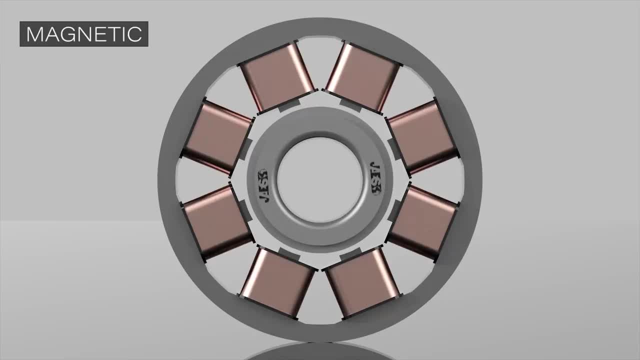 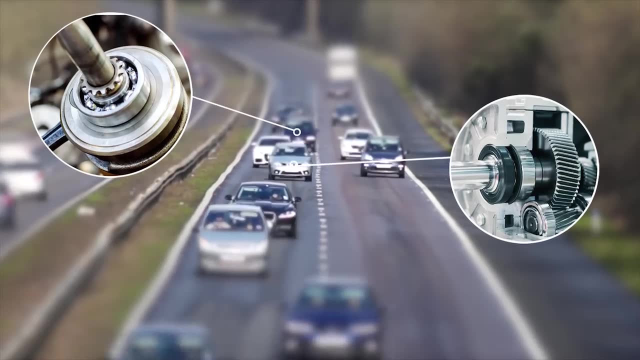 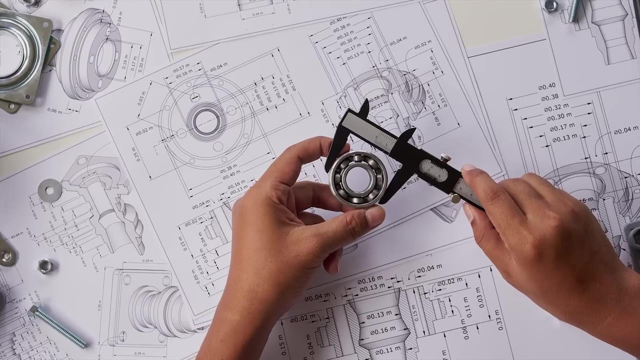 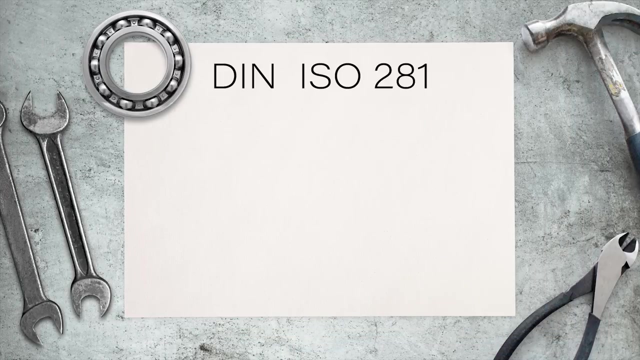 even in extreme temperatures, but one should always pay attention to the curry temperature of the magnetic system. Bearings are one of the most important things for the machine, most used mechanical parts and there are many varieties of them, so it is important to consider the area of use when choosing the right bearing. the reference standard for bearings is din iso. 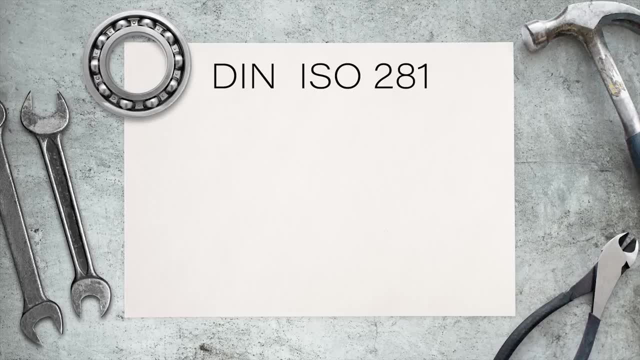 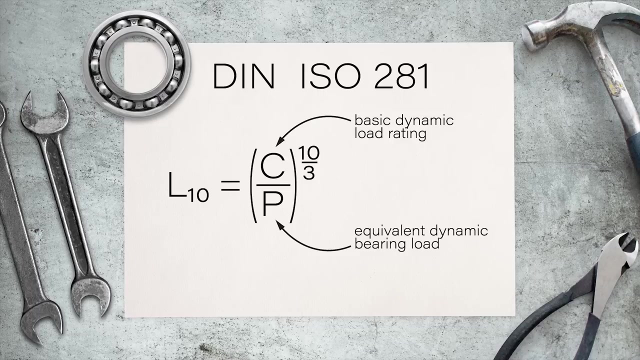 281, which provides a formula for calculation of bearings durability. given the basic dynamic load coefficient of the bearing c, the equivalent dynamic load p and the specific coefficient, which is 3 for ball bearings and 10 thirds for roller bearings, this allows us to obtain the durability of the bearing expressed as millions of turns. the equivalent load p is: 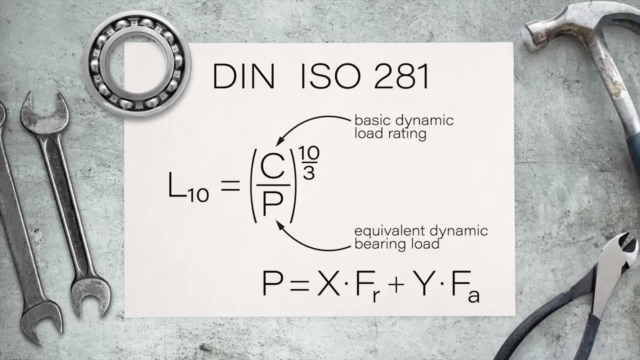 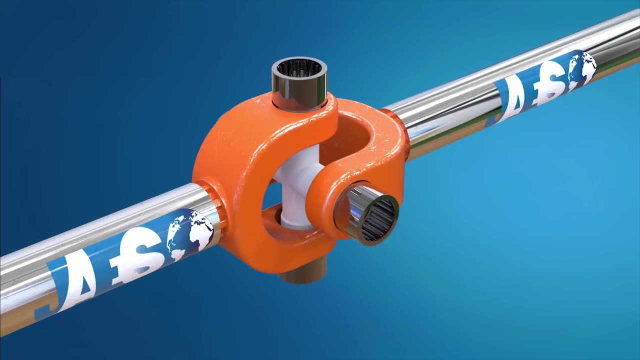 calculated on the basis of the radial and axial load which act on the bearing the. The coefficient of basic dynamic load is instead determined by the fatigue behavior of a significant lot of equal bearings. Bearings are always used on shafts and joints to keep them in position without causing high friction.